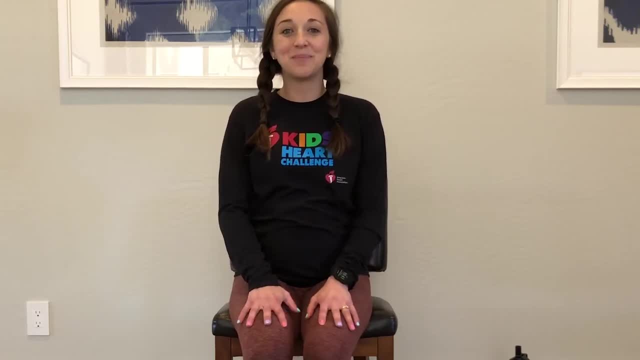 We're going to do that two more times. Go ahead and inhale through your nose. so that means: breathe in, Exhale, breathe out One more time. inhale through your nose, Exhale through your mouth. Just a little bit of breathing techniques helps us calm our minds Now. 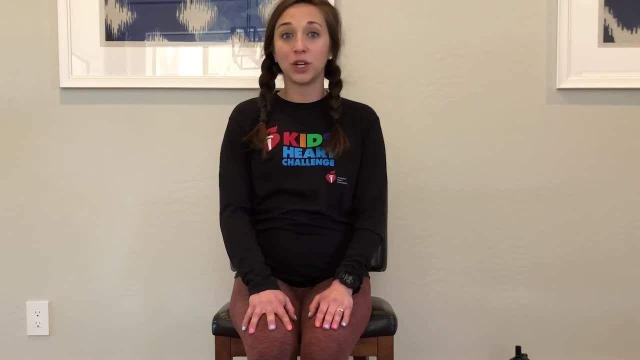 we are going to begin by rolling our shoulders. So go ahead and take your shoulders all the way up to your ears, all the way back down to your back, like a big shoulder shrug. Let's go ahead and do that again while still breathing Again. this should take out the tension in our shoulders. 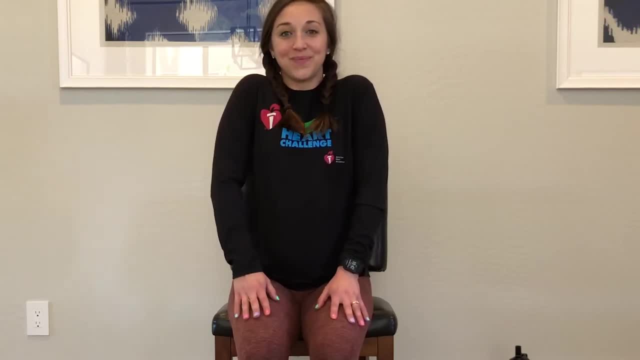 Let's do it one more time: Exhale- All right with our chair. we are going to begin with some stretches. Let's do it one more time: Exhale- All right with our chair. we are going to begin with some stretches. 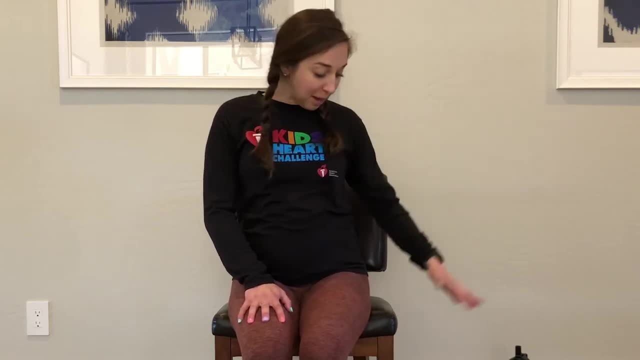 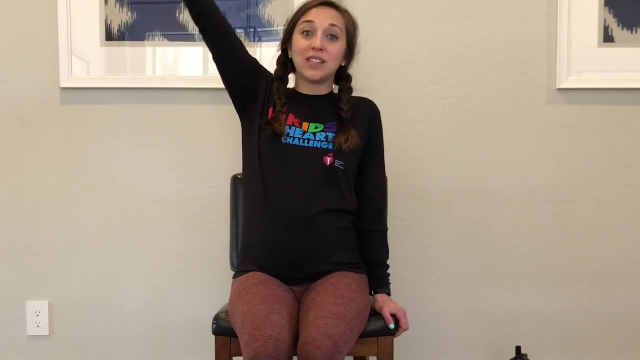 So, first and foremost, what I want you to do is take one of your hands and place it on the side of your chair. okay, Now we are going to take our opposite hand and put it up towards the ceiling and stretch over towards that hand that's on the chair. 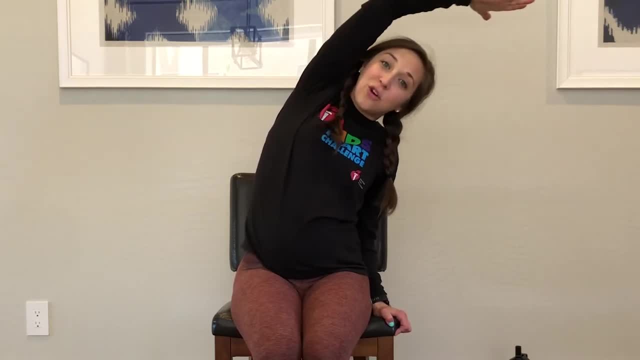 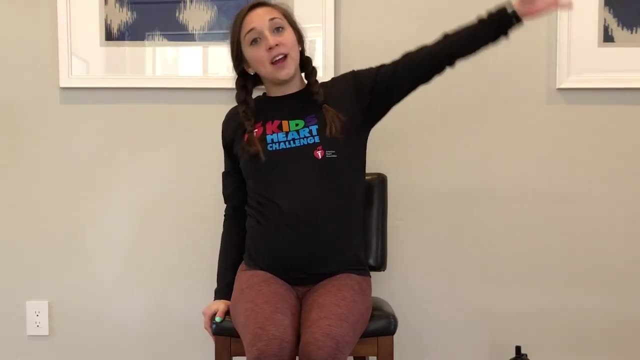 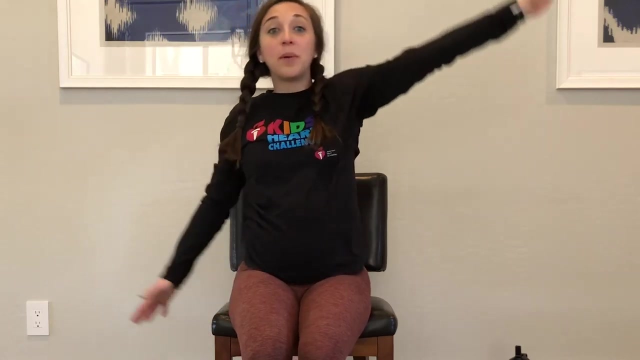 Make sure you guys are supporting yourself so you don't fall. Let's go ahead and switch that out. Take the opposite hand, put it on the chair and we are going to stretch towards the other side. Begin to rainbow back and forth with your hands side to side. 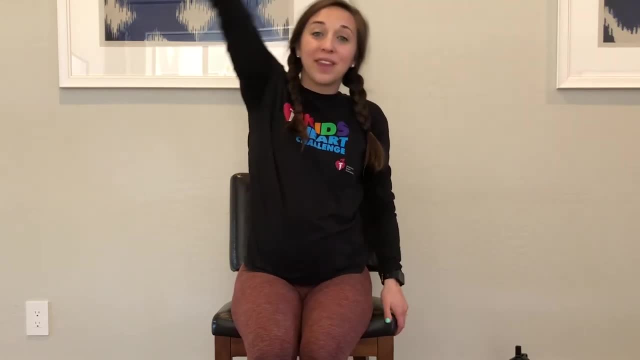 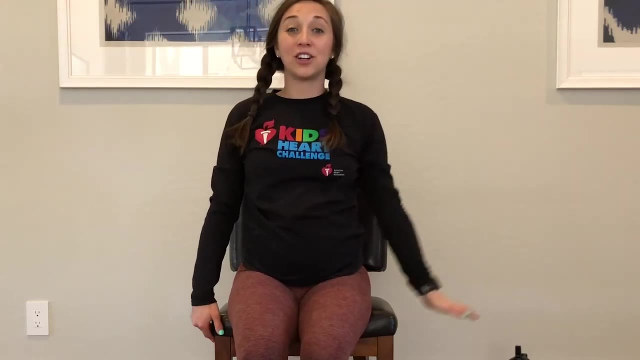 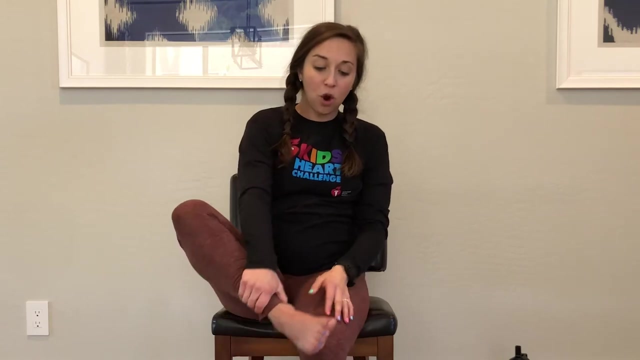 You should feel this stretch in your side body Should feel really good. Never should hurt. All right, our next yoga pose. we are going to take one of our legs and we are going to put it over our other. thigh, okay, Make sure you keep your foot on the side of your leg. 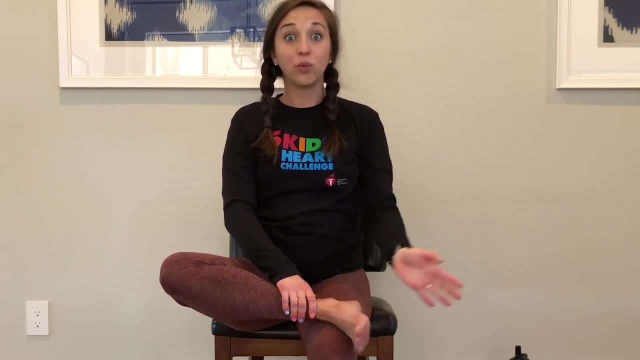 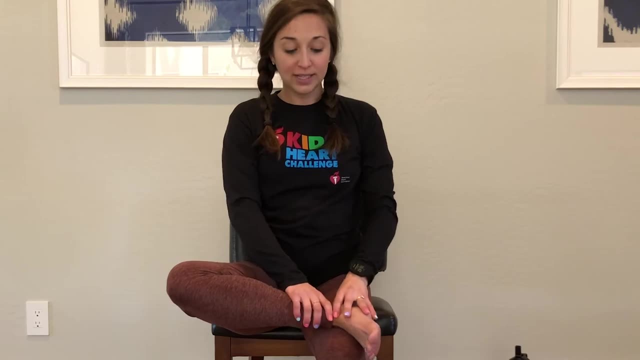 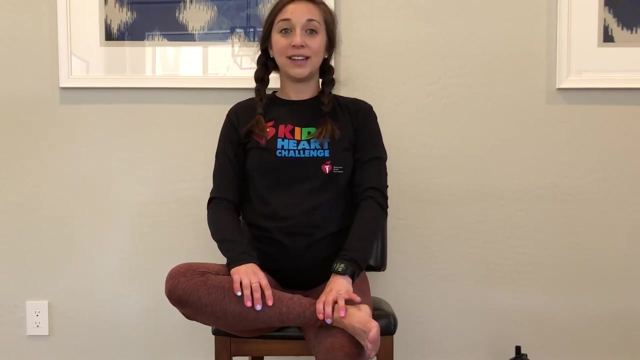 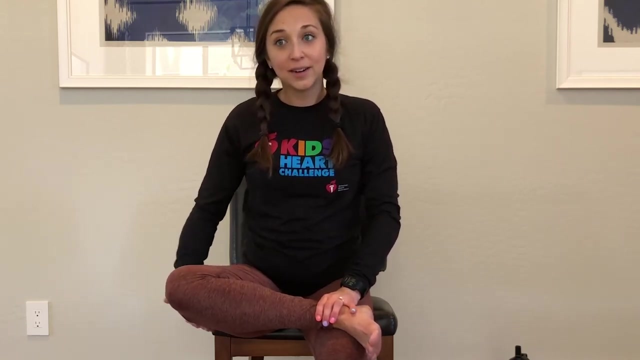 Foot not pointed but reflexed, okay, So that will protect your knee. Make sure you guys are sitting up straight. Make sure your ankle is at the very end of your other thigh. Sit up straight And if you want a little bit more sensation, you can kind of lean forward and you'll feel that right here.